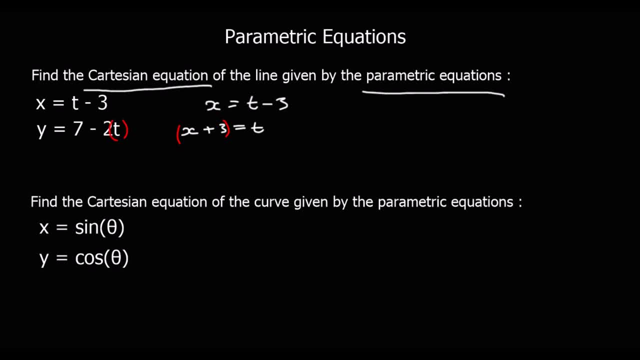 substitute it in for the T in the Y equation, So that will give me Y equals seven minus two, substituting X plus three for T. So now I've eliminated T And we can just simplify this a bit by expanding the bracket Seven minus two, X minus six, And we can write it in the form: Y equals MX. 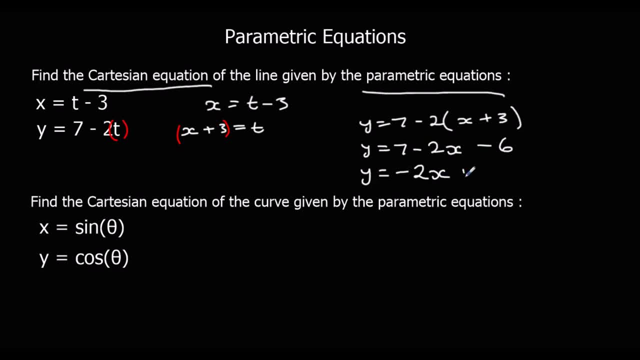 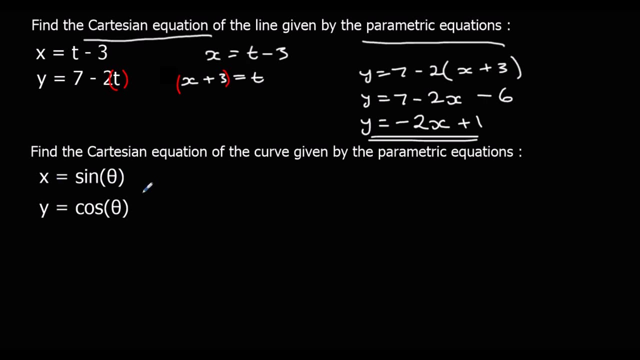 plus C, So Y equals minus two, X plus one. So there's our Cartesian equation When we have trigonometric equations. so here are parameters, theta. So we're going to eliminate theta. We've got X equals sine theta, Y equals cos theta. We use the identity sine squared theta. 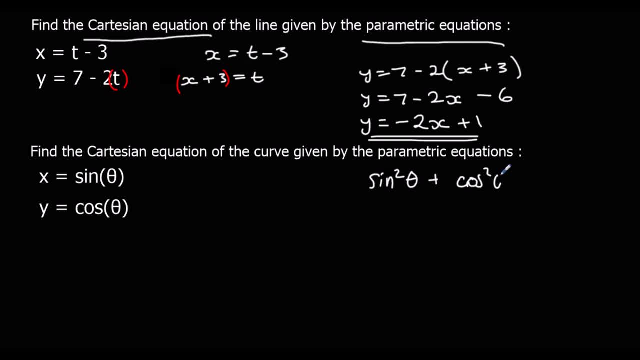 Plus cos squared theta equals one. So we rearrange this to make it sine squared theta, Rearrange this equation to make it cos squared theta and substitute them both in to the identity. So if we square both sides, we get X squared equals sine squared theta. If we square both sides here, we have Y squared, equals cos squared theta. 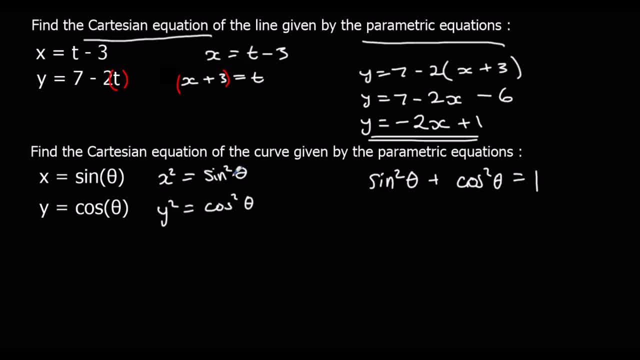 So we've got sine squared theta. So I can substitute sine squared theta for X squared. I can substitute cos squared theta for Y squared And I would have eliminated theta. So sine squared theta is X squared, Cos squared theta is Y squared equals one, And there's our equation. So with trigonometric, 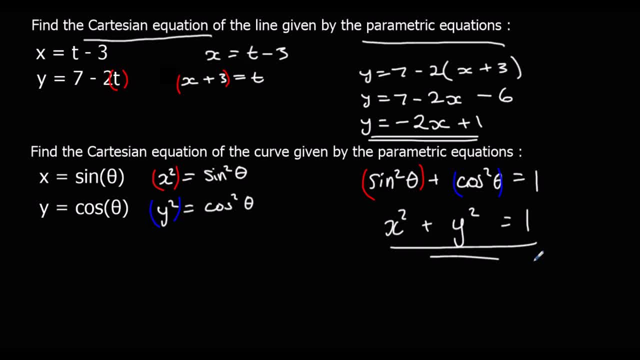 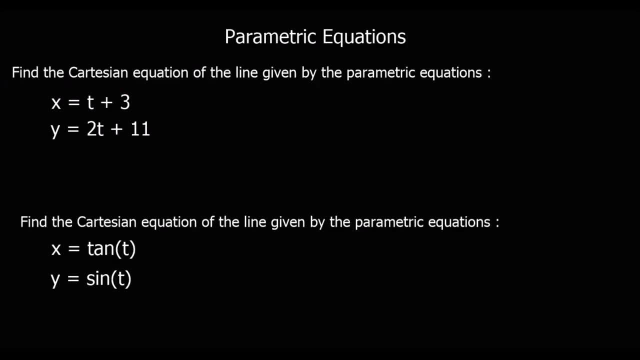 equations, trigonometric, parametric equations. we use the identities to eliminate the parameter. Okay, two more questions here. So find the Cartesian equation of the line given by the parametric equations: X equals T plus three and Y equals two T plus eleven. 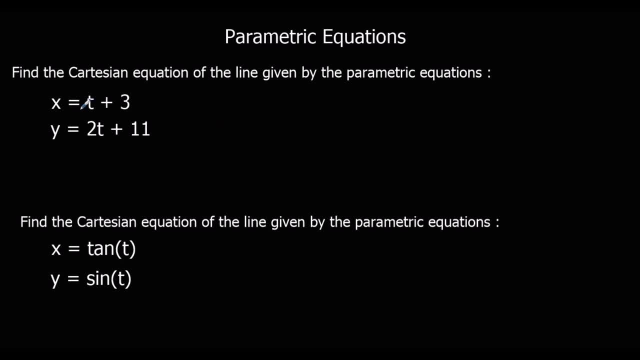 So for this first question we're going to make the top equation equal to T. So take away three from both sides, subtract three. we get X minus three equals T. So we just substitute X minus three for T on the second equation and we would have eliminated T. 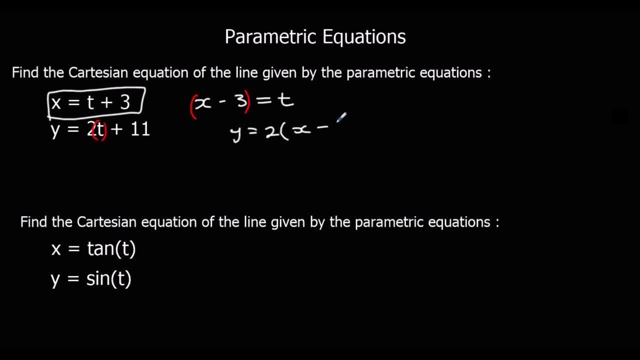 So Y equals two times X minus three plus eleven. We expand the bracket to simplify it. We've eliminated T. at this stage We've got a Cartesian equation, But we're going to simplify it. So 2x minus 6 plus 11, which is 2x plus 5.. 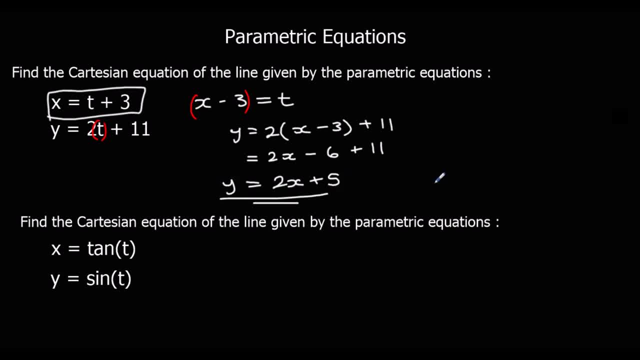 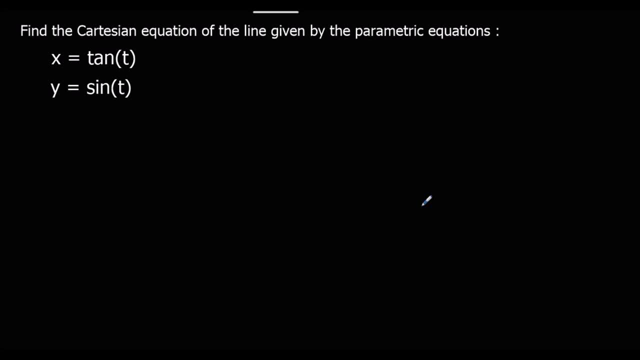 So our Cartesian equation is: y equals 2x plus 5.. The second equation here is a trigonometric one. So we've got two equations, two trigonometric equations, And with trigonometric equations we almost always use the identity sine squared t plus cos. squared t equals 1 to eliminate our parameter, to eliminate t. 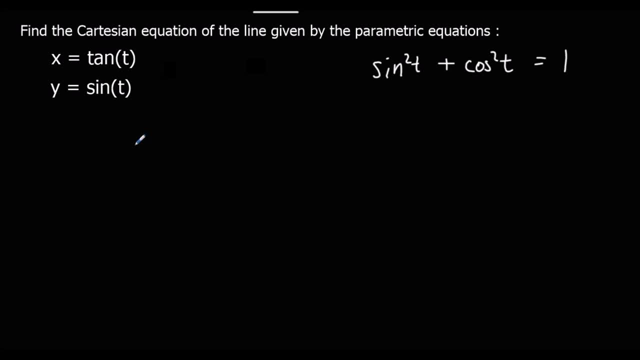 So we're going to need one of these equations to be sine squared t equals, the other one to be cos squared t equals, and then we can substitute them in. So for the y equation, that's easy If we square both sides: y squared equals sine squared t. 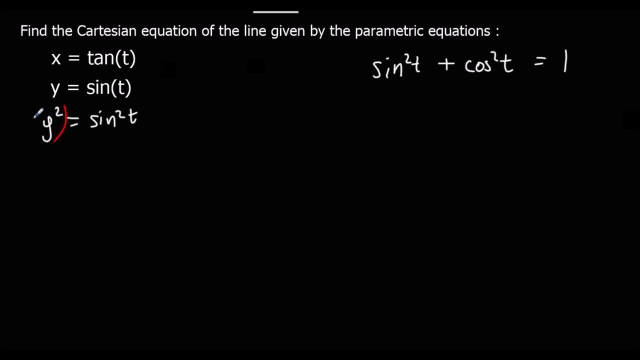 So we can grab that y squared, substitute it in for sine squared t and we would have eliminated the sine squared t. For the x it's a bit harder. So we've got x equals tan t. How can we make that cos squared t? 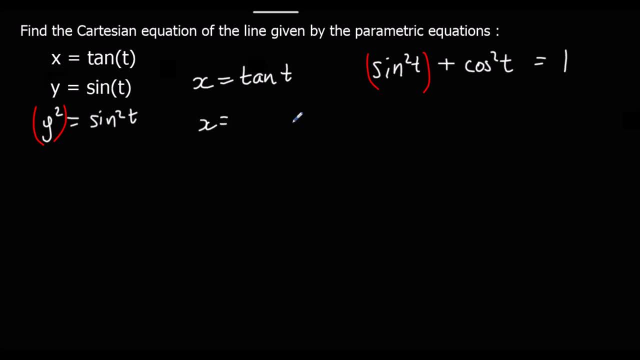 So we're going to have to change x to get a cos. We'll change it to sine over cos. So now we've got a cos t. If we multiply both sides by cos t, so x cos t equals sine t and divide both sides by x, cos t equals sine t over x, and then square both sides, so we've got cos squared t. 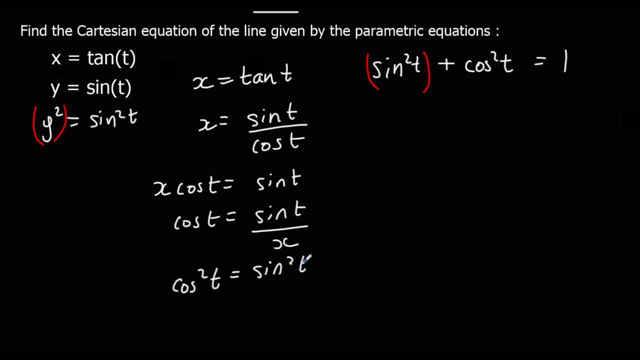 Cos squared t Is sine squared t over x squared, So we can substitute this in for cos squared t. So if we substitute them in now, we've got y squared plus sine squared t over x squared equals 1. But we've still got a t. 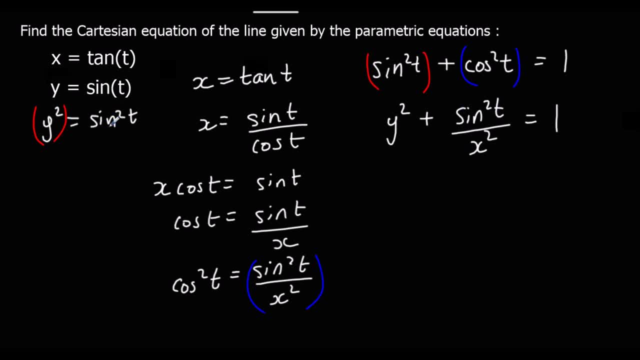 We've still got sine squared t, but we know sine squared t is y squared, So we can substitute y squared in there. y squared equals no y squared plus y squared over x squared equals 1.. So we've eliminated t. 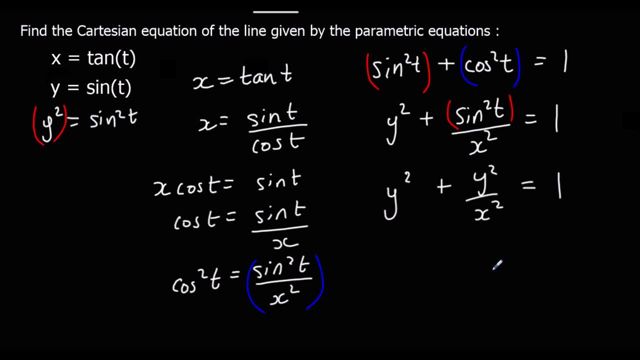 So we've got our Cartesian equation. We could leave it there or we could try and simplify it. If we were asked for it in the form y equals f of x, we'd have to rearrange to make it yx, Which we could do in this case. 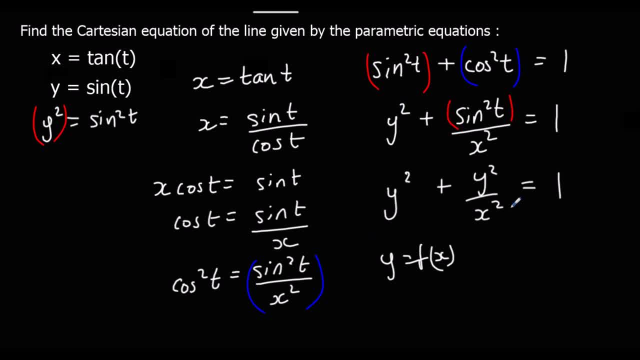 But we'll leave it there. We'll leave it as it is. So we've eliminated our t, So we've got our Cartesian equation. We weren't asked to put it in a specific form, so we'll leave it as it is. 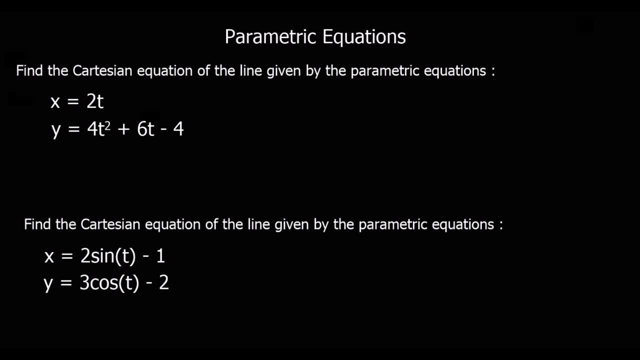 Okay, two more questions. So pause the video, give these ones a go and then press play when you're ready to go through. Okay, Okay so. So the first set of equations we're going to make an equation equal to t. 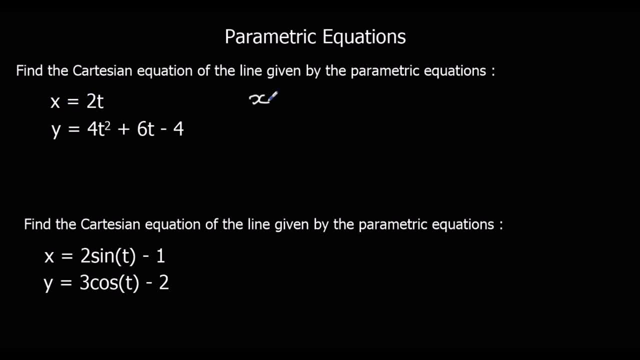 So if I half both sides of the top equation, x over 2 equals t, And then we're just going to substitute that in to our second equation. So y equals 4 times x over 2 squared, plus 6 times x over 2 minus 4.. 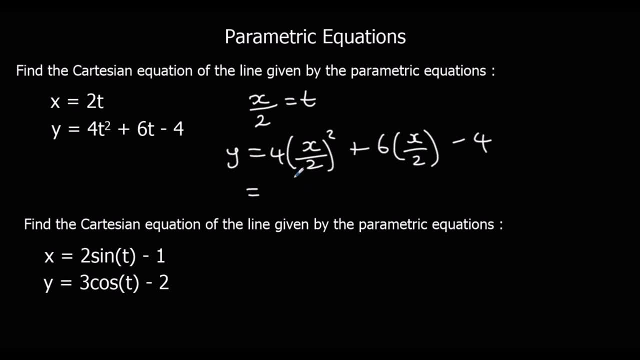 So x over 2 squared. I'm going to scribble it up here: x over 2 squared. So that means x over 2 times x over 2, which is x squared over 4.. So 4 times x squared over 4 is just x squared. 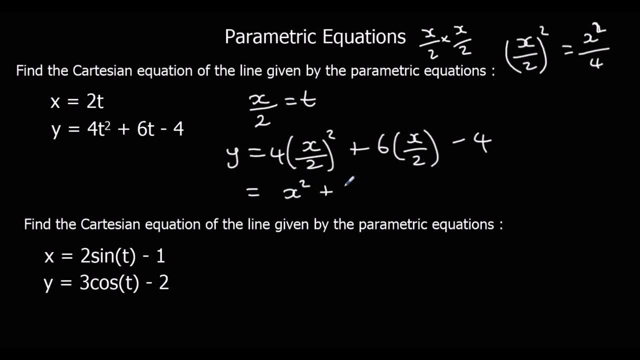 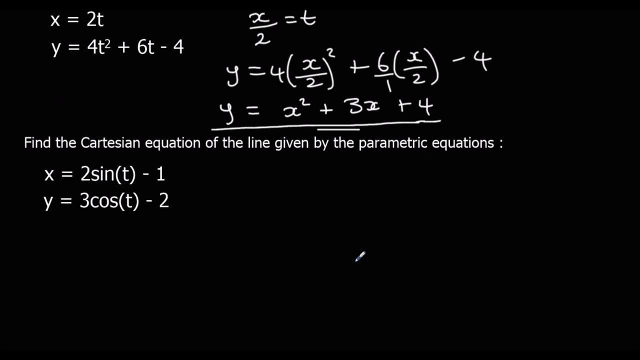 6 times x over 2.. 6 over 2 is 3, so 3x Plus 4.. So y equals x squared plus 3x plus 4.. For the second one, again we've got a trigonometric one. 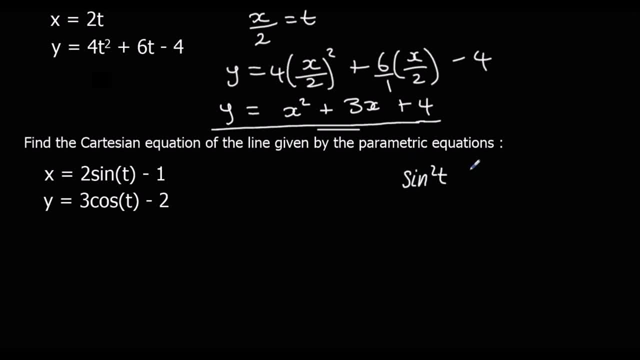 So we'll use the identity sine squared t plus cos squared t equals 1.. And we'll rearrange one of the equations to be sine squared t, one to be cos squared t, and then substitute them in. So for the x one we plus 1 to both sides. 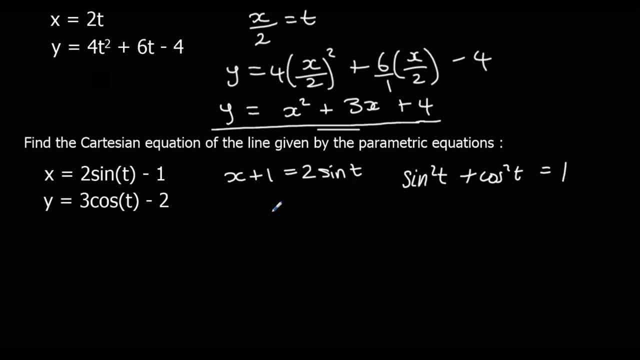 x plus 1 equals 2 sine t. Divide both sides by 2.. So x plus 1 over 2 equals sine t. And then square both sides, So x plus 1 squared over 4 equals sine squared t. So that's that part done. 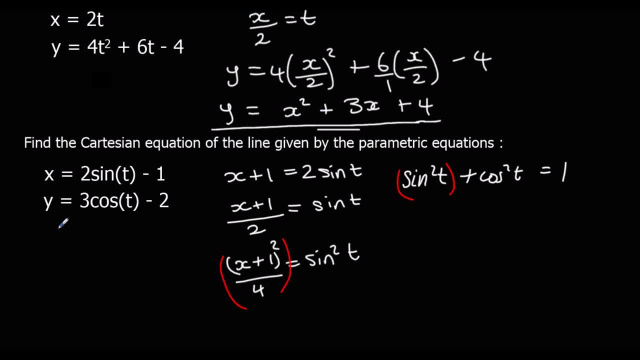 And then for the y same thing. So plus 2 to both sides, y plus 2 equals 3 cos t. Divide both sides by 3.. y plus 2 over 3 equals cos t, And then square both sides. 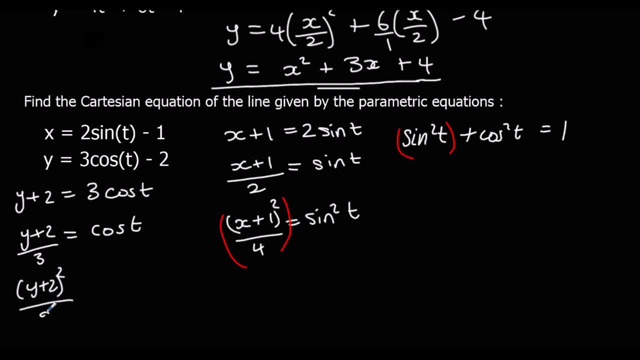 So y plus 2 squared over 9 equals cos squared t, So we can substitute that one in as well. So we have x plus 1 squared over 4, plus y plus 2 squared over 9 equals 1.. I think it's best if we leave it like that. 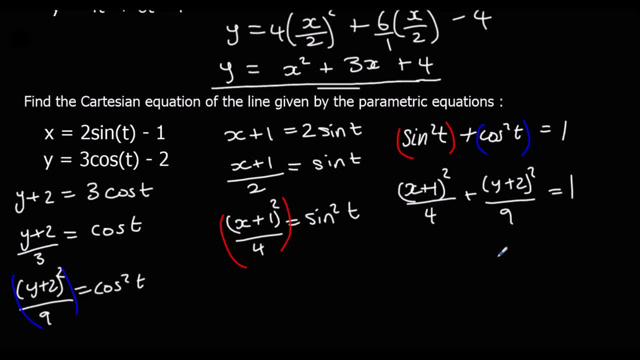 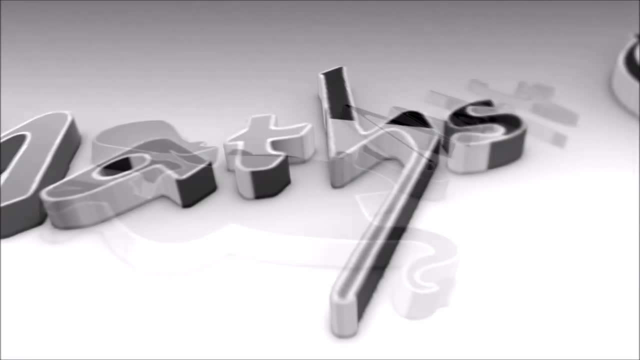 So we've eliminated our t, We've eliminated our third variable. So that is our Cartesian equation. So let's go to the next dhx equation before we go to numbers and subdivisions. So, overall, 45 is our integral, This is our k squared. Noi please stand. Okay, Alright, Hold on for 3 seconds. Okay, 1 over 2.. Alright, 1 and 2..